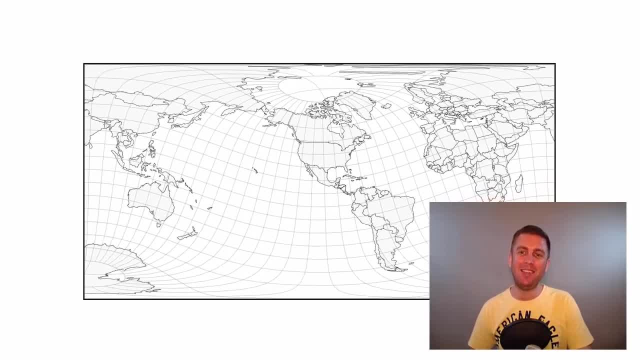 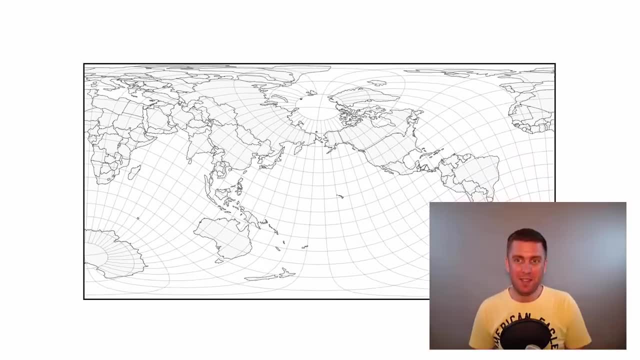 Hey guys, what's cracking? This is Chris here at Mango, and today I'm bringing you a video on map projections. Now I know what you're thinking: map projections, oh, this is going to be all about maths and geometry and complicated equations, but don't worry, this is going to be a beginner's guide. 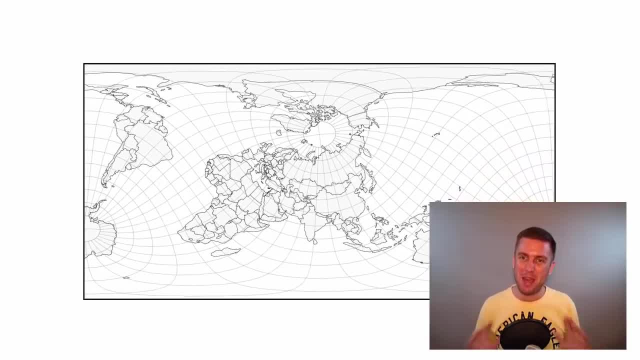 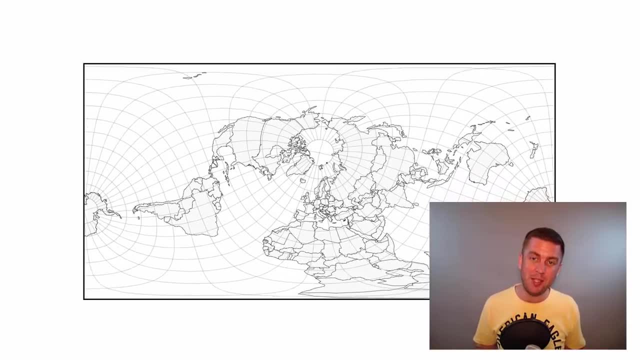 so we're going to be gentle with you and we're going to ease you into the basics of map projections and hopefully, by the end of this video, you'll firstly understand what a map projection is and, more importantly, you'll understand what impact it has on your map applications, especially. 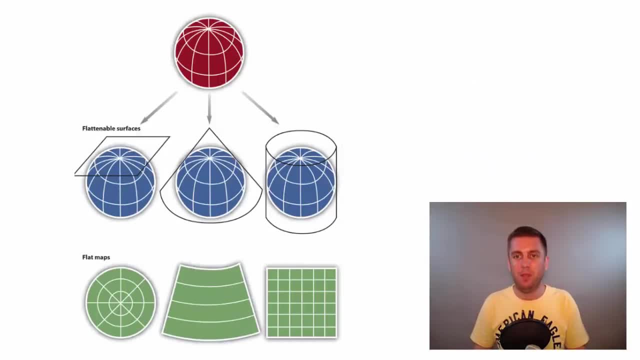 in terms of measurements of distance and area. So what's a map projection? A map projection, as you can see on screen at the moment, is the process of transforming a spherical object into a two-dimensional flat surface. So that usually means taking a sphere, in this case the 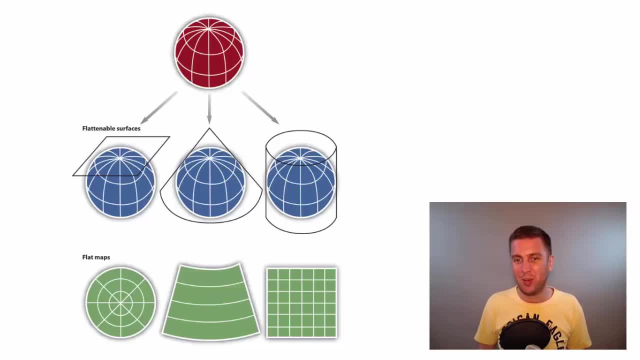 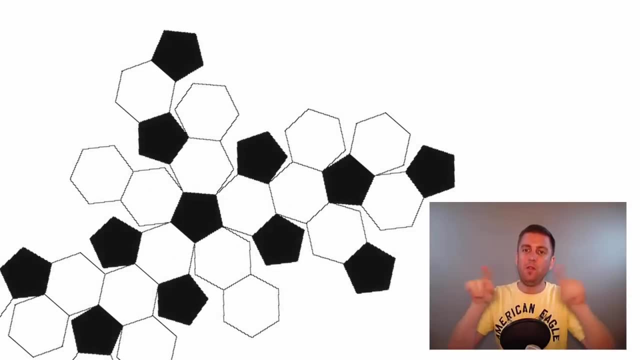 earth and transforming it into a flat square or rectangle. Now, as you can imagine, if I took a football and I began cutting it up with a knife and tried to flatten it out, it wouldn't fit together perfectly into a rectangle or a square. So a 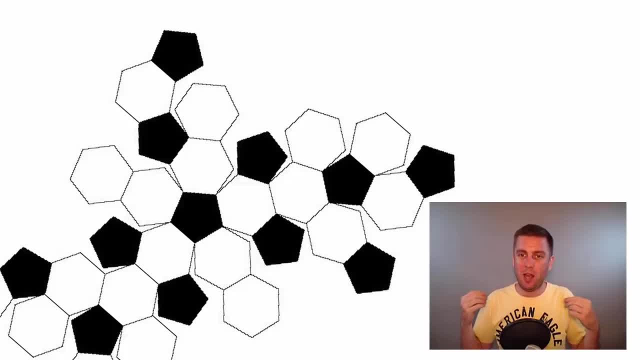 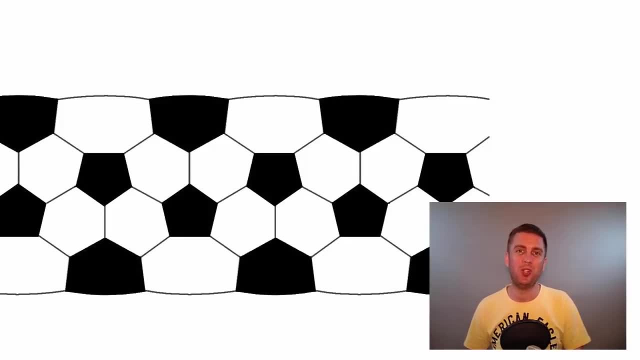 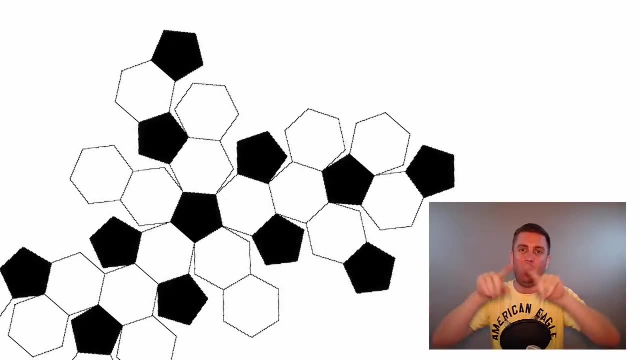 projection is a mathematical equation that tells a mapping system how to fill in those gaps and how to populate the entire rectangle. When it comes to map projections, distortions are the name of the game. Think back to our football. if we slice the football up and we try and spread it out into a rectangle in order. 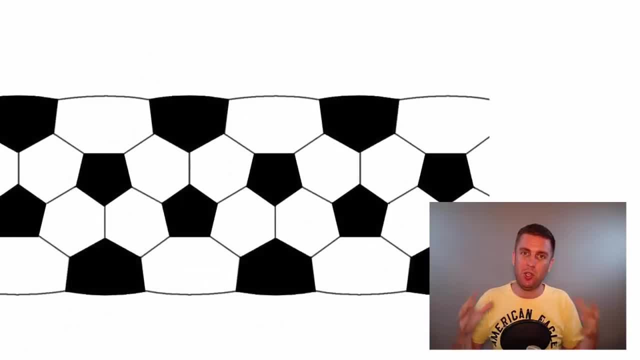 to make that shape, we're going to have to introduce some distortions of the picture that was contained on the surface of that sphere. We're either going to lose the distances- they're no longer going to be accurate- or the shapes will be inaccurate, or the areas will be inaccurate, or the directions. 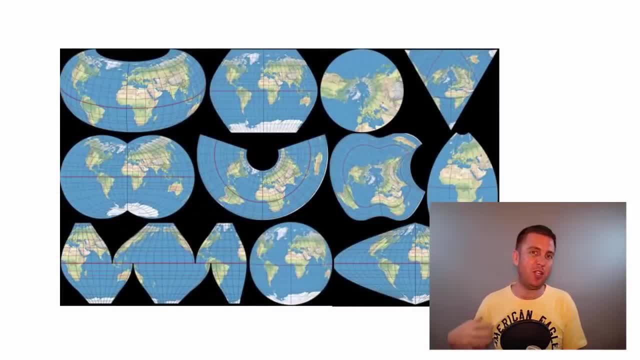 will be inaccurate. So when creating a projection, it's always a question of compromise. Which of these attributes are we willing to compromise? Some projections try to maintain the correct distances between locations on the surface. others try to maintain the area or the shape or the direction, and many projections 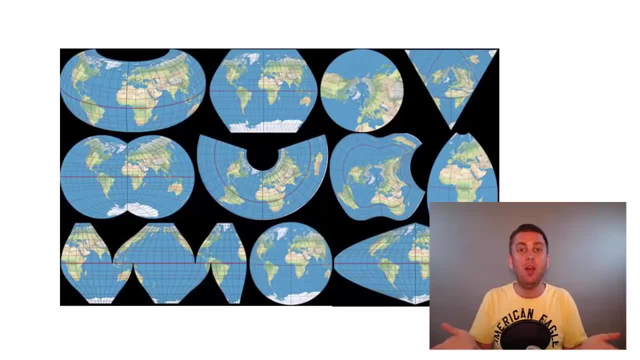 try to find a sweet spot, a balance in all of these variables that gives the most accurate visual representation for a specific area on the globe. that's why you often see projections that are for individual countries, states or regions, so let's take a look at one of these. 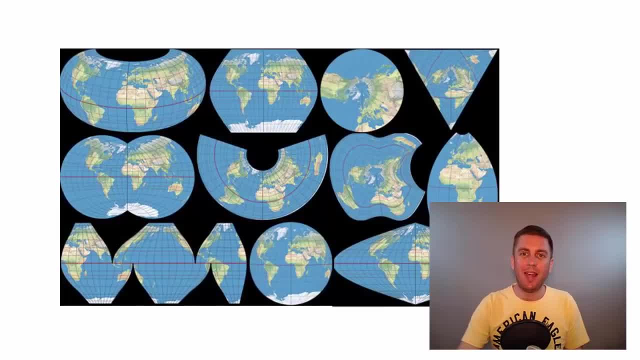 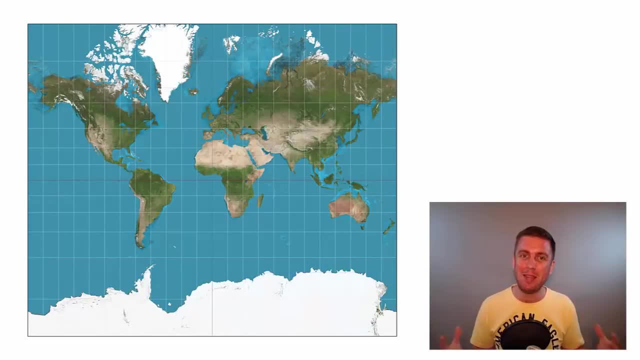 projections and look at the distortions that it introduces. today, we're going to be looking at the WebMakator projection now. i've chosen the WebMakator projection not because it's the best projection by any means, but because it's probably the most viewed projection of all map projections. 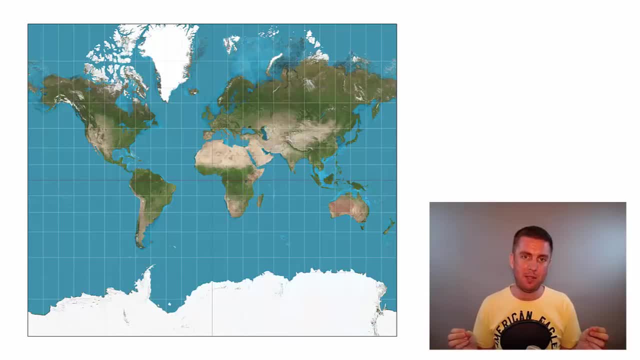 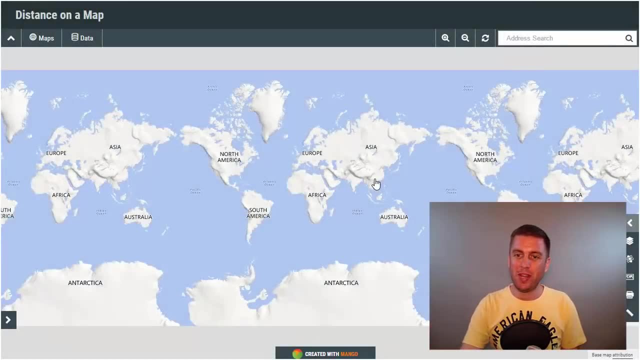 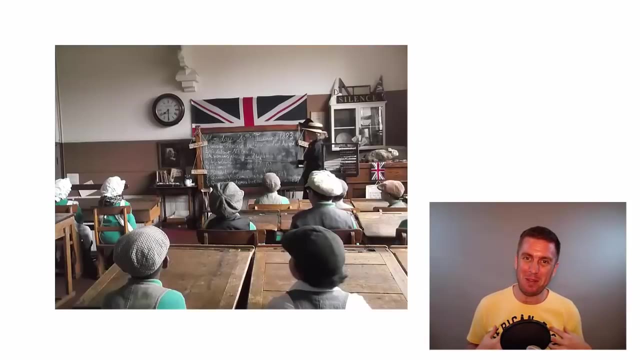 today, because this is the projection that's used by web mapping systems such as Google Maps, Bing or the base maps that you see on Mango. so the map that you see on screen at the moment is a WebMakator projection of the globe. now, for those of you who are digital immigrants, like myself, 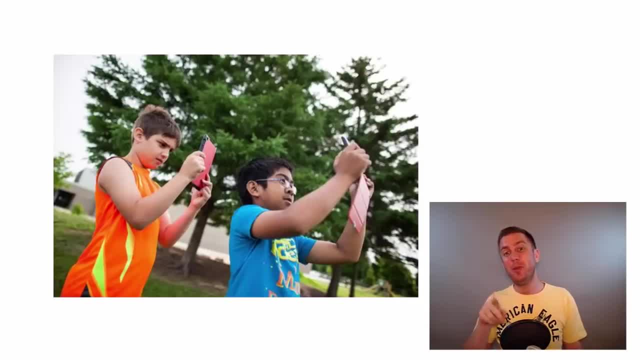 and learn a little bit about webmkator in the past. you probably know that webmkator is an overseas app from Japan and all the states around the world. now geography from a textbook rather than Google Maps. you'll be looking at this map and you'll notice that there's one or two things wrong. First of all, 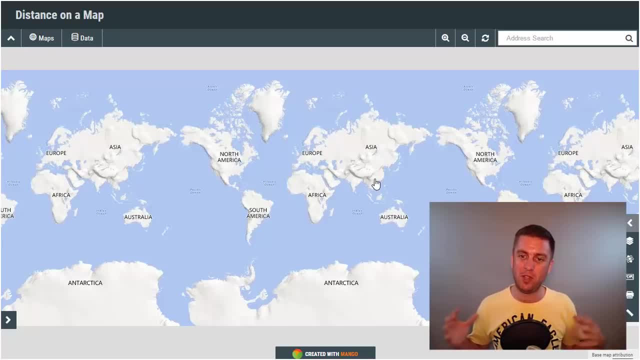 Antarctica seems to have a larger landmass than the rest of the the rest of the continents combined and secondly, Greenland looks to be at least as large as Africa. This is because the Webb Mercator projection creates very large distortions at the poles, because it stretched the sphere out into a square. 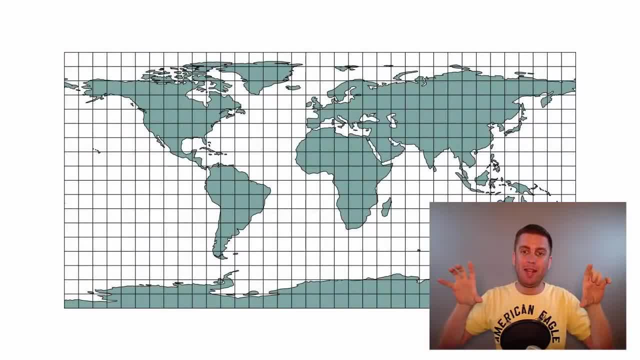 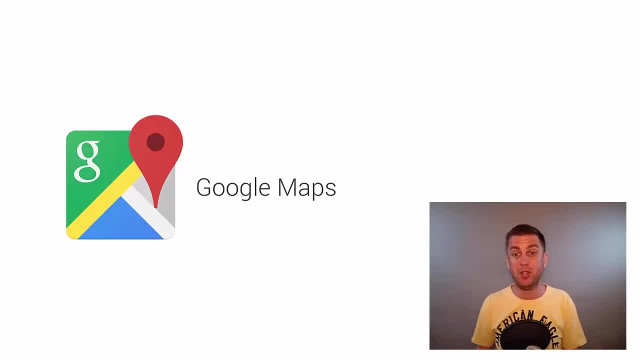 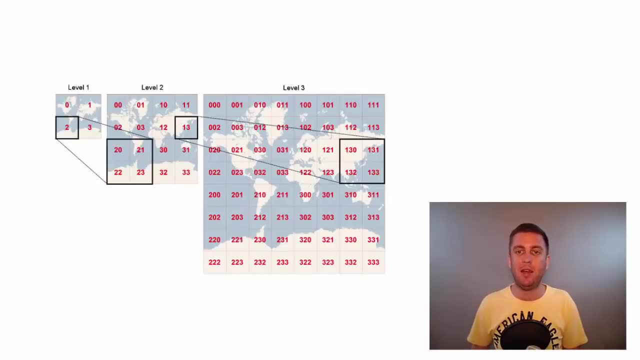 whilst naturally that sphere wants to be stretched into a rectangle shape. Now there's a lot of technical reasons why Google, who originally created this, this projection system, chose to do that. mainly, it was to do with storage efficiency and the speed which they could send map tiles across the internet. 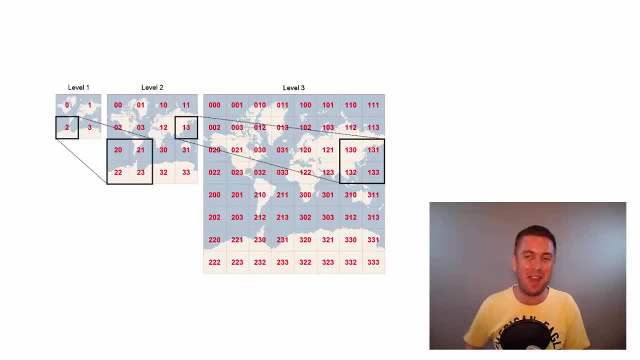 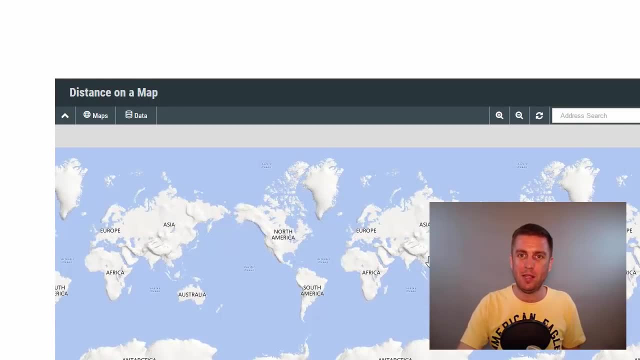 but I'm not going to bore you with the technical details of that today. maybe we'll save that for another video. Okay so, but the main thing here is these distortions at the pole. so, as we see here, Greenland is the same size as Africa. so, as the image shows here, the image on the left- 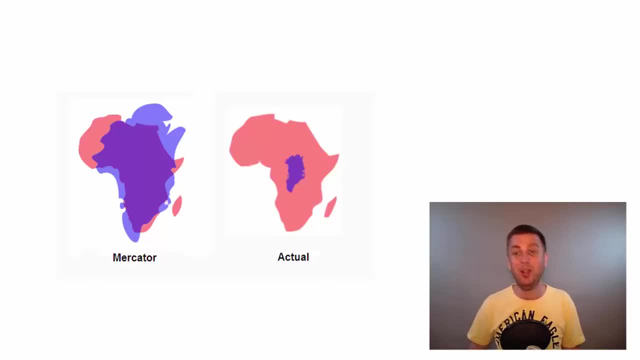 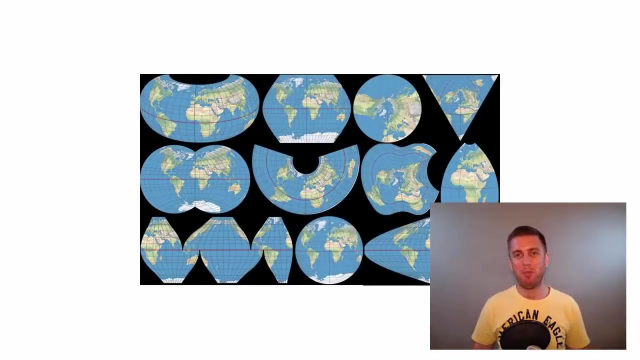 shows Africa compared to Greenland using the Webb Mercator projection. as we can see, they're nearly the same size. on the right, we see how big they are in comparison. in reality, as you can see, Greenland is a fraction of the size of Africa. so now that you understand projections and you also have an 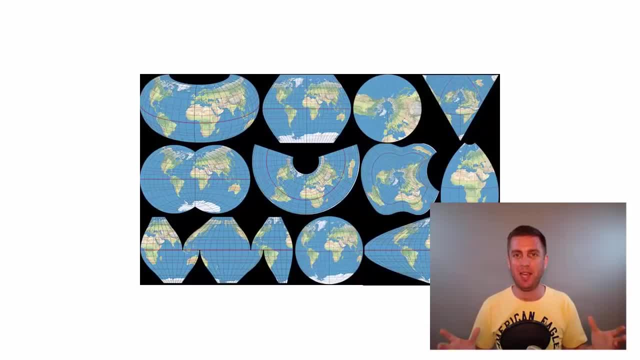 understanding of the distortions that they can introduce in your map visualizations. You're probably wondering: what practical impact does that have? what impact does that have on me when I'm interacting with a map application? or if you're a maker of maps or web maps, what impact does it have for your users? I think one. 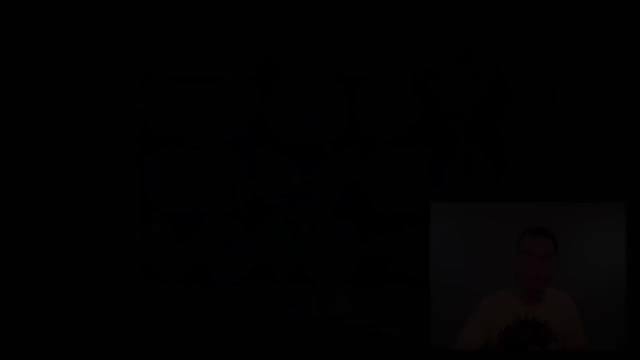 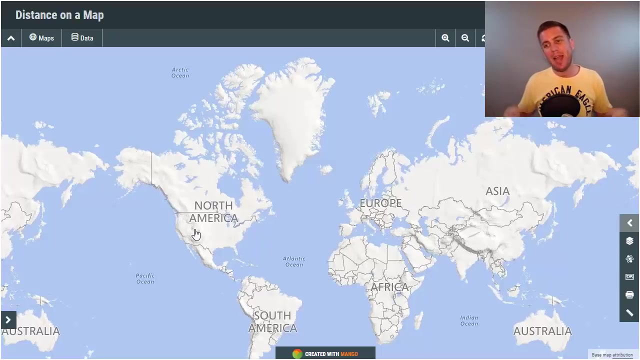 of the best ways to demonstrate this is by using circles and radiuses. so we'll go back here to this base map on Mango that's in the Webb Mercator projection again, and what I'm going to do is I'm going to draw a couple of circles on the 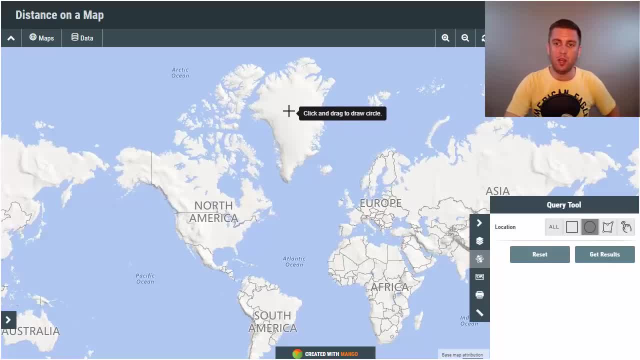 map and using a radius tool. so I'm going to draw one circle up here near Greenland and let's make the circle say 500 kilometers wide. okay, so on this map, at the moment, that 500 kilometer wide circle, in terms of my screen size, is probably about five centimeters wide. so 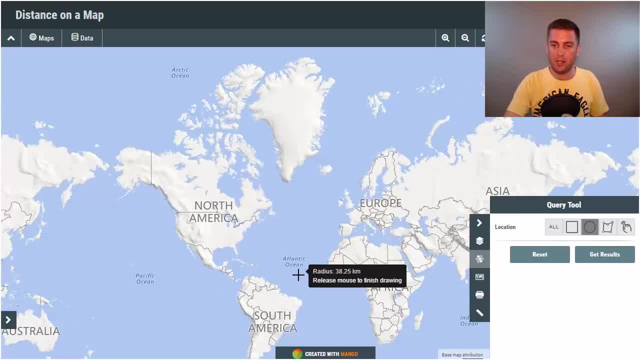 let's see what happens. if I draw the circle again close to the equator, we can see that now 500 kilometers is is smaller than the tip of my little finger. so there's a big difference between what the area of a 500 kilometer circle looks like near the equator. 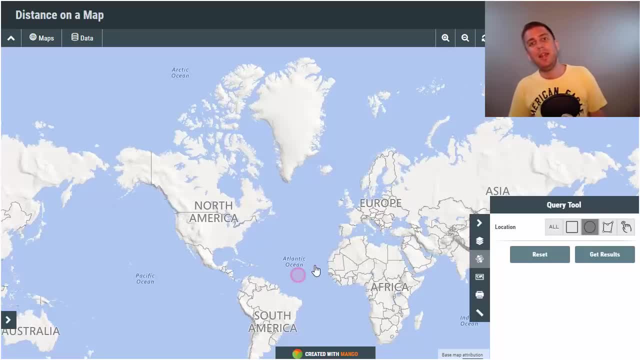 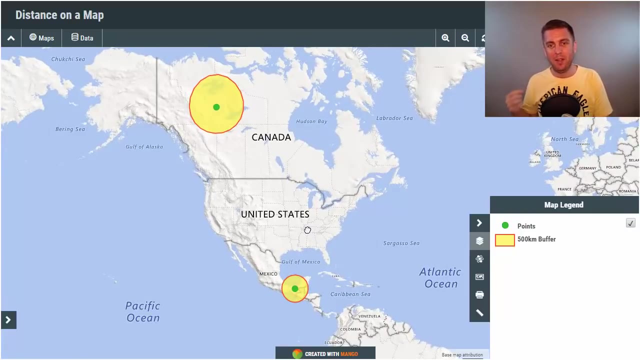 and what it looks like near Greenland. So how can that impact your tools and your queries and your measurements? Let's look at a layer that I've prepared on this map previously. So this is a map where I place two points, one in Mexico and one in northern Canada- and once I place the points, I use. 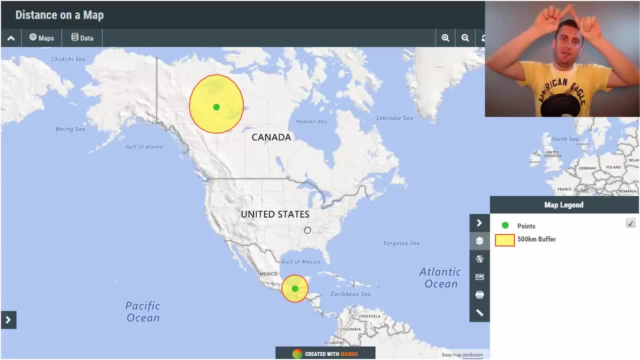 the buffering tool to draw a circle exactly 500 kilometers around each of those individual points. So the two circles that you see on screen- the yellow ones on the surface of the true earth, are exactly the same size and they have an exact radius of 500 kilometers from that point. 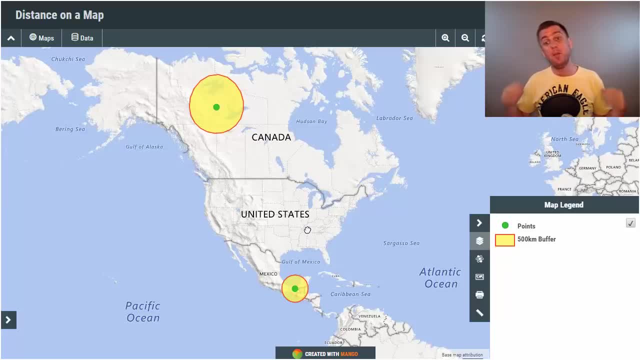 But looking on the map, you can't see that. It's obvious to see here that the circle in Mexico looks much smaller on this map and the circle in Canada looks much larger. What's more is the circle in Canada, as you can see, is no longer a perfect circle. 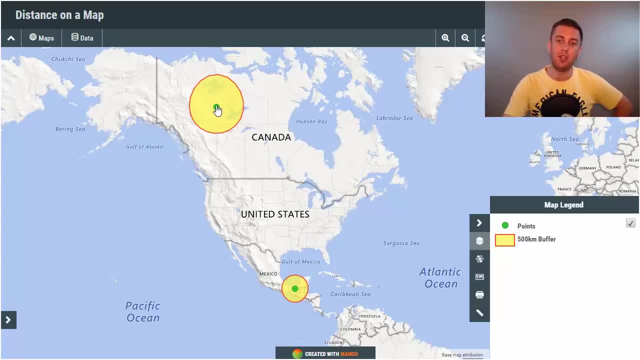 It's starting to resemble an egg shape and we can see that the dot, the green dot here, which is the center point of that circle, looks like it's much closer to the southern edge of the circle than it is to the northern edge, But the reality is that every edge around this circle is exactly 500.